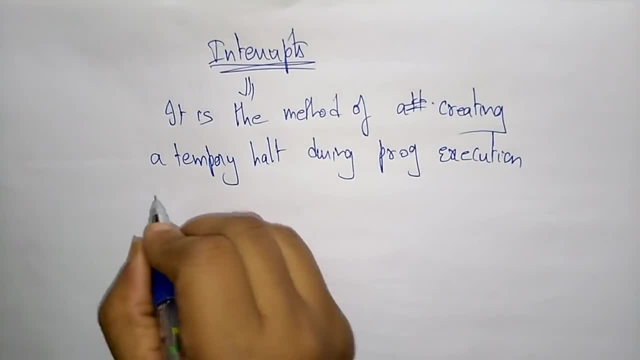 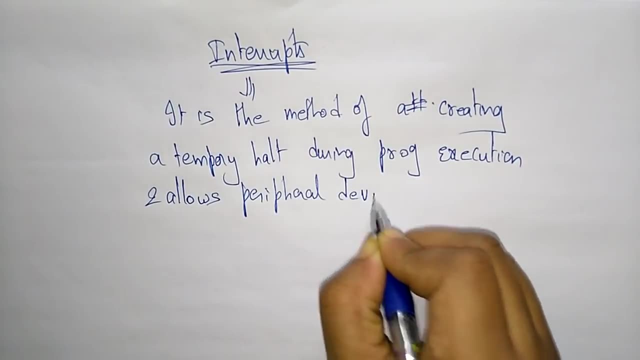 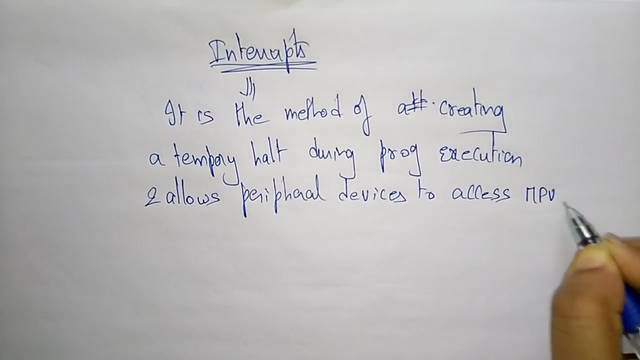 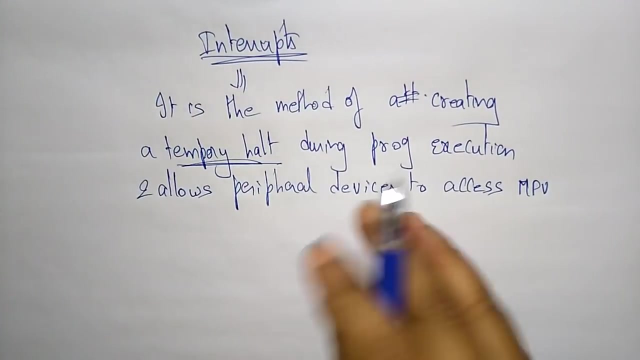 So it is just a temporary halt during program execution and allows peripheral devices to access microprocessors, to access the microprocessor unit. So that is an interrupt. Interrupt is nothing, but it is a process of creating a temporary halt. You just, it is a temporary halt during program execution and it is allowing the peripheral 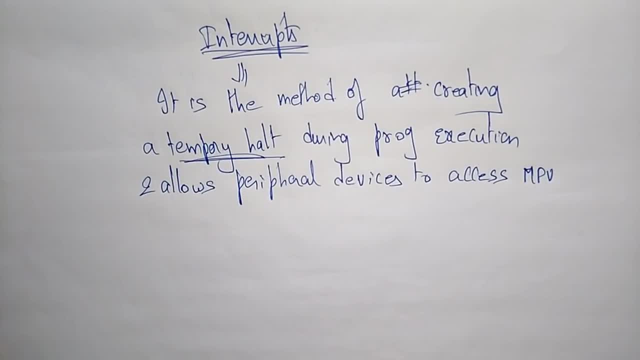 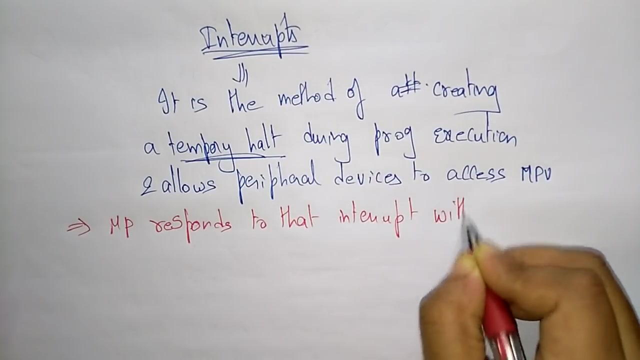 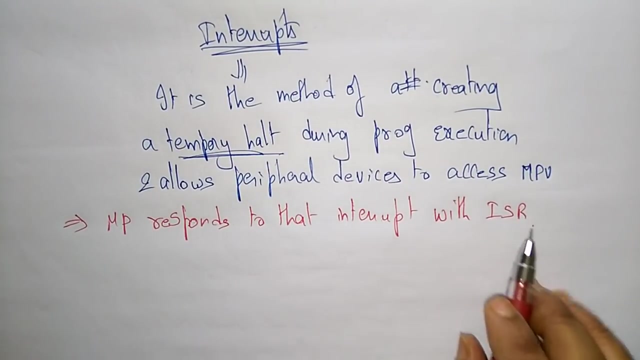 device, the external devices to access the microprocessor unit. So here the microprocessor unit responds, a microprocessor unit responds. responds to the interrupt with interrupt service routine. So when the microprocessor unit is respond, so with the help of the interrupt service routine. So, which is a short program, Interrupt. 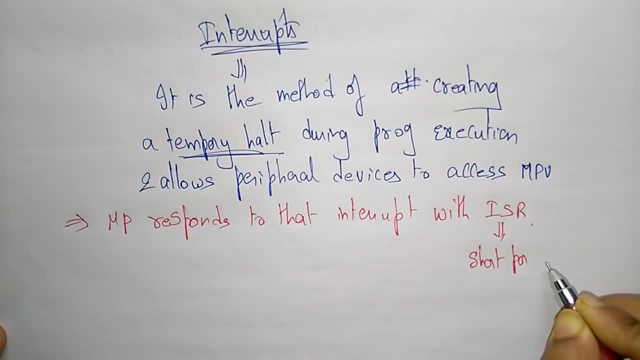 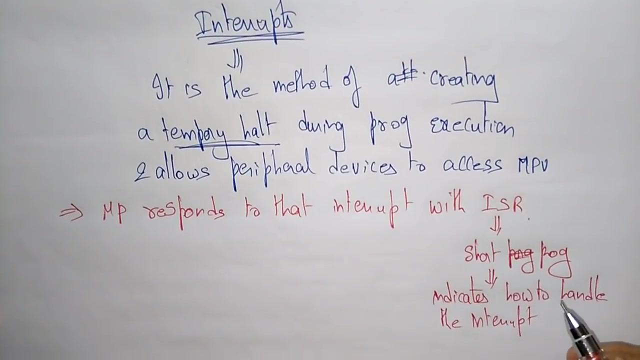 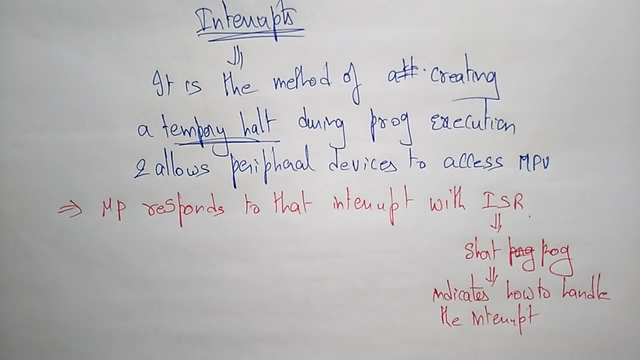 service routine is nothing but it is a short program to instruct the microprocessor on how to handle the interrupt. Short program indicates how to handle the interrupts, So means it is just a program. the interrupt service routine is program. it is a saying to the universal which interrupt would have to be taken based on their priorities, which interrupt is having the highest? 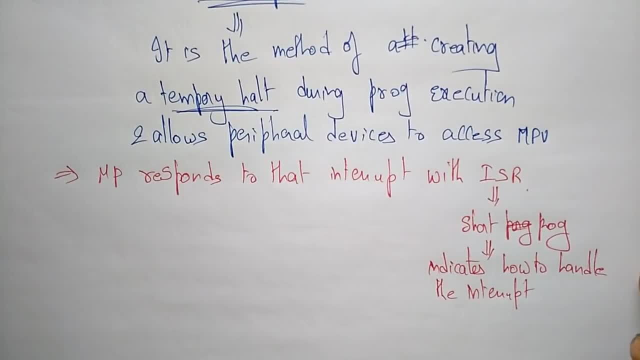 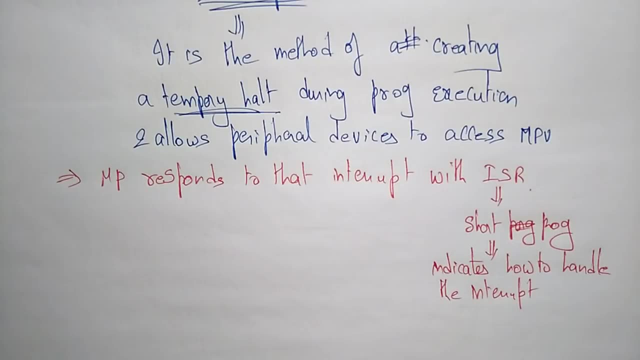 to priority. It indicates how to handle the interrupts, the microprocessor. So interrupts are useful when interfacing IO devices, water dispenser, devices with low data transfer rate, like keyboard or in mouse, in which case case pulling the device waste variables processing time, so actually the processor jumps to a special 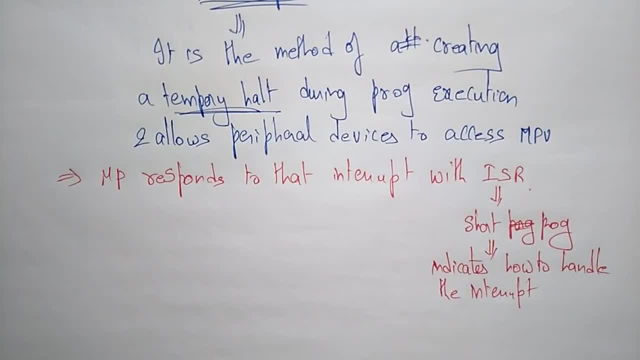 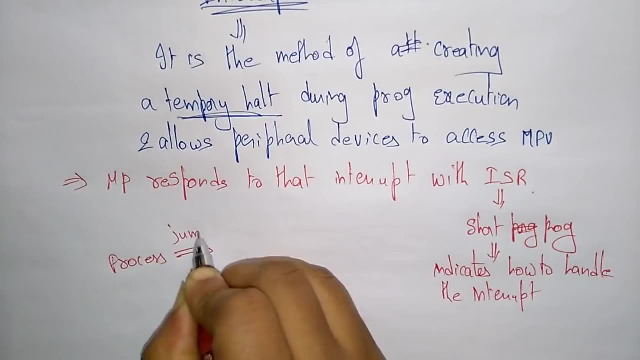 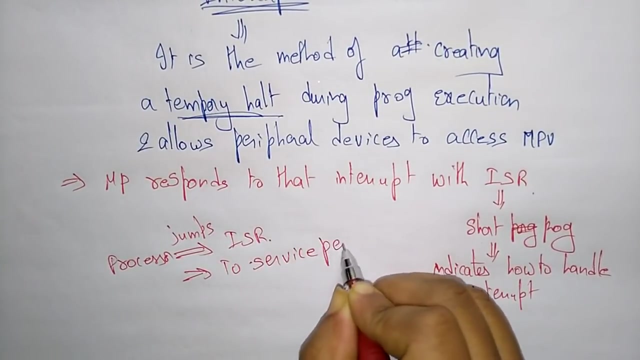 program, that is the interrupt service routine to service the peripherals. so the mainly whenever the interrupt the processor, the microprocessor jumps to interrupt service routine, why it jumps to the interrupt service routine to service the peripherals. okay, to service peripherals. so whatever the request, that is, peripherals or requesting the microprocessor so to service. 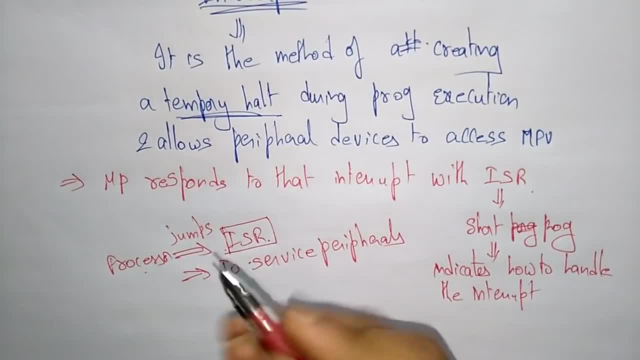 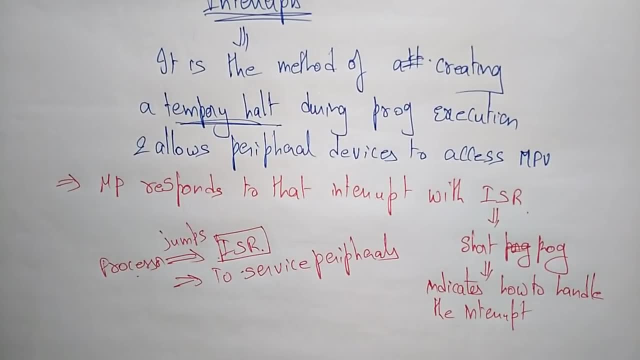 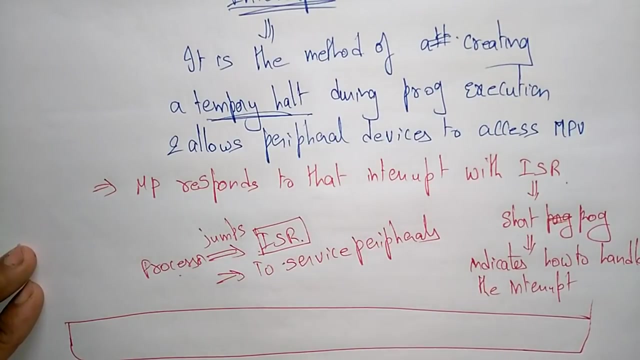 those peripherals the processor will jump to interrupt service routine to take the interrupt request from the peripherals. so after the processor service this peripherals, the execution of interrupt program continues. so just like, suppose here I am writing one, suppose the processor is doing some main program. it is working on program, a main program. so 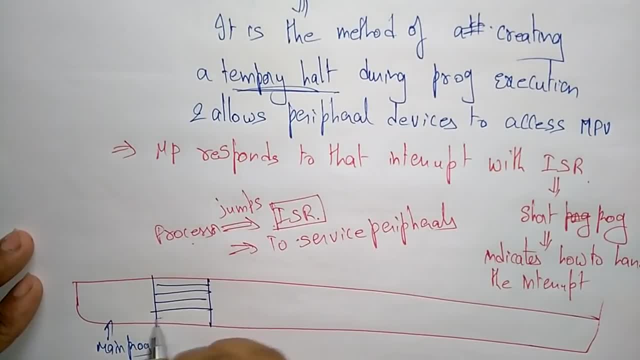 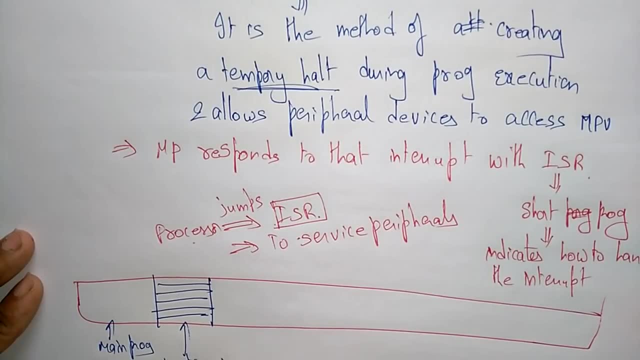 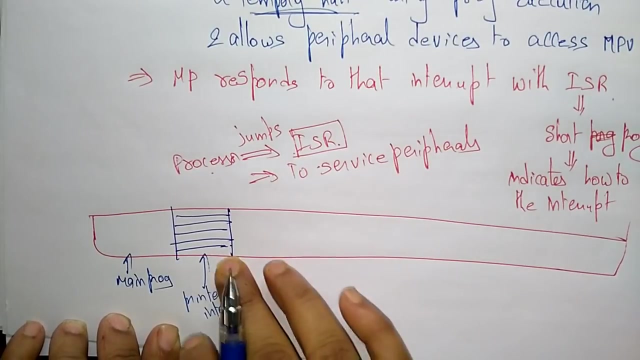 suddenly an interrupt is occurred. so interrupt it means the printer requested. printer interrupt means if you want to print some data, okay. so the printer interrupt is occurred to the processor. so now the controller jumps to that interrupt service routine. the processor jumps to that interrupt service routine. the processor jumps to that interrupt service routine. so the controller. jumps to that interrupt service routine to service the interrupt. so after completion of the interrupt service again the pro processor continue with the main program. at some time again the interrupt occur. so now the processor jumps to the interrupt service routine to service the peripherals. so next time it comes to the a modem interrupt is occurred, modem is requesting. 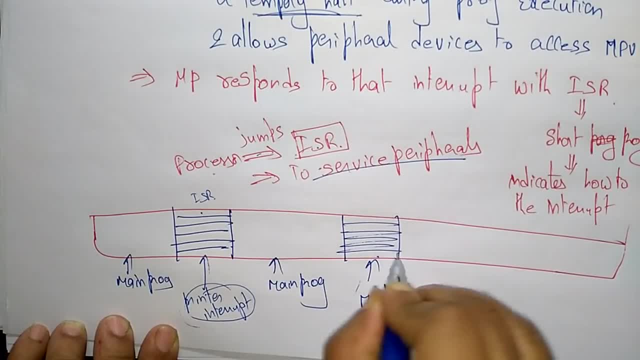 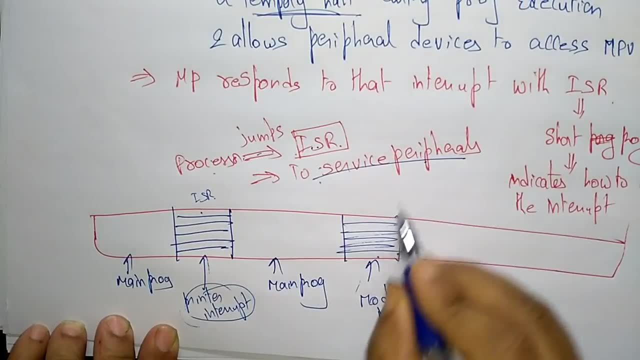 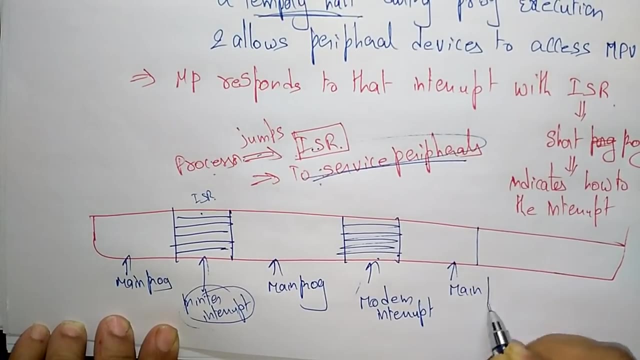 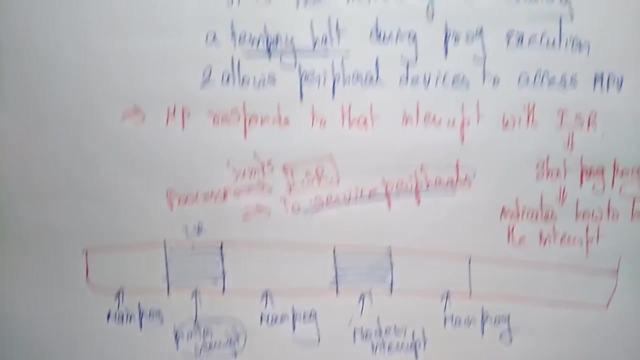 to work on some data by the processor. so the controller, it stops the main program and it jumps to the interrupt service routine to service the peripherals. after the completion of this peripherals request, again continue with the processor, continue with the main program. so this is how the interrupt service routine will help in the program. so there are different types of 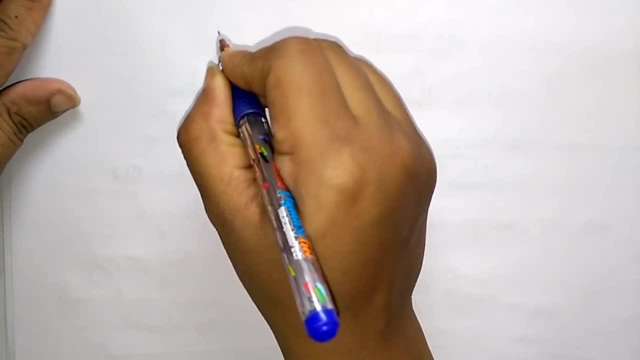 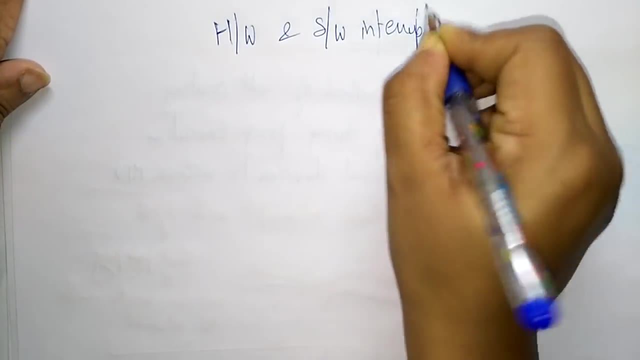 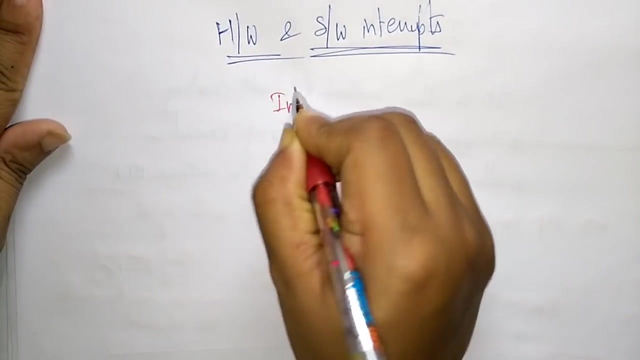 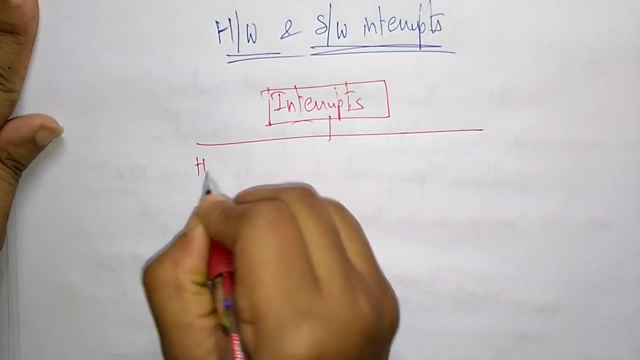 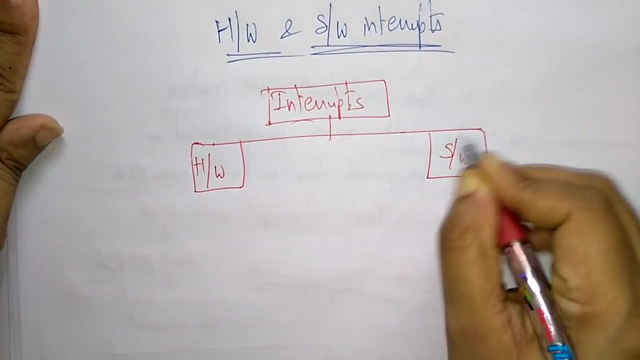 interrupts that are present in 8086 microprocessor, so those divided into hardware interrupts and software interrupts. so those are two types of interrupts present in 8086 microprocessor: hardware and software actually interrupt is there. so interrupts is of two types: hardware interrupt and software interrupt. so again, this hardware interrupt is of maskable interrupt. 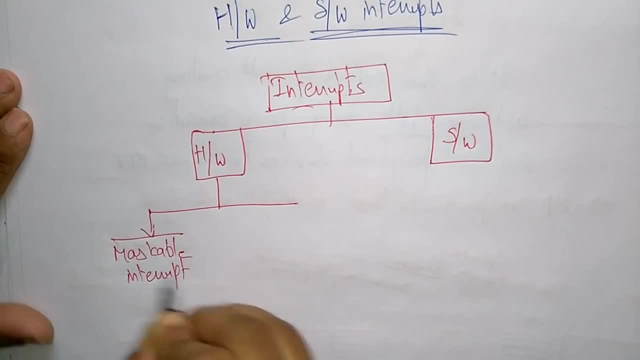 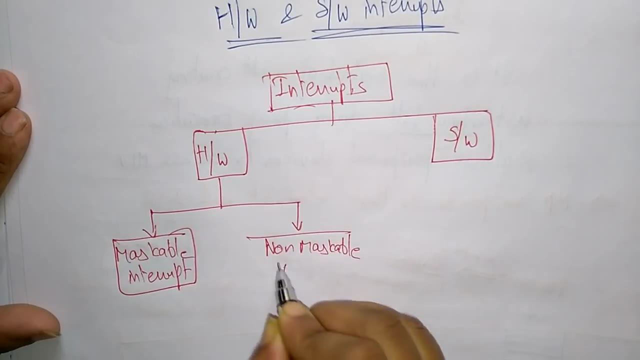 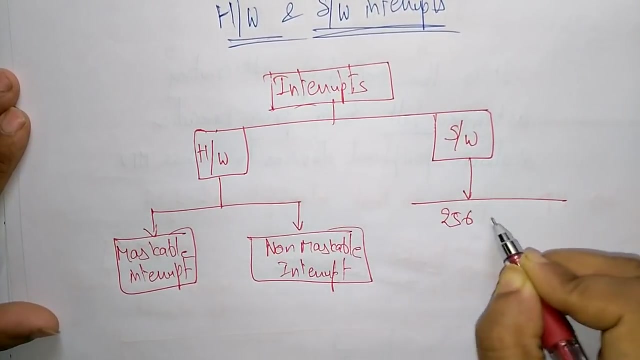 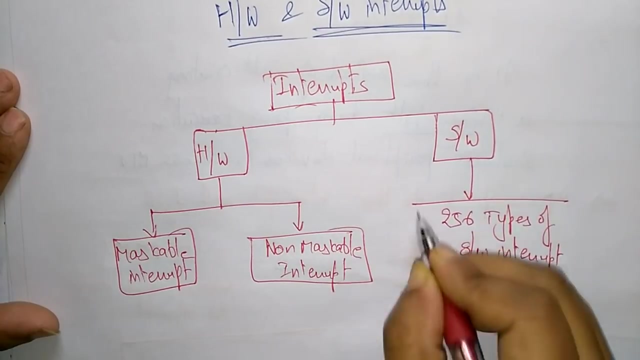 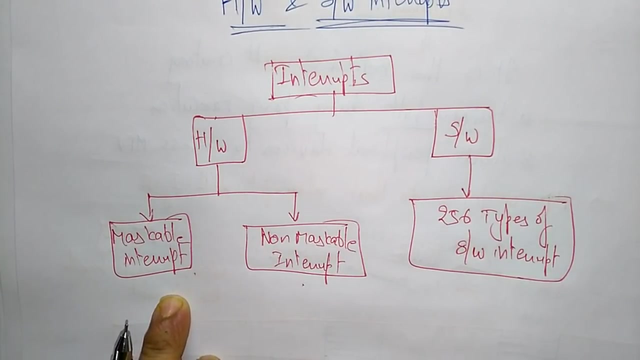 non-maskable interrupt. software interrupts all totally. 256 types of interrupts will be there for software. okay, hardware is only two types: maskable or non-maskable. maskable means means having least price. whenever the maskable interrupt is occur, the processor can mask this and it can continue with. 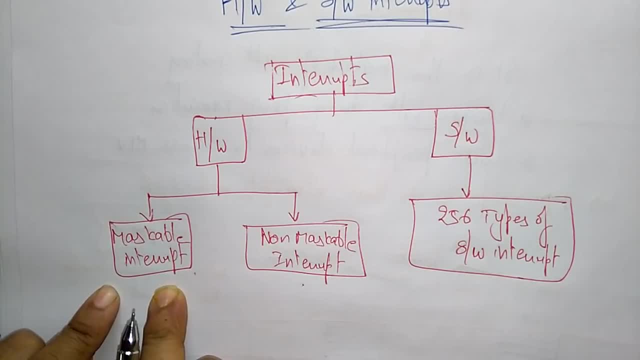 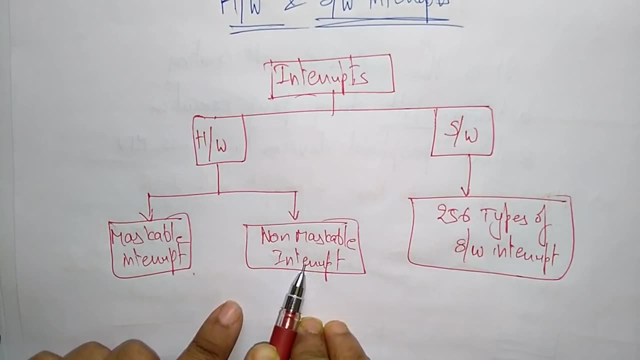 the main program. after the completion of the main program it takes the maskable interrupt and non-maskable means you can't ignore that. you have to take that request of whatever the non-maskable interrupt is sending this signal. so the processor first has to complete the non-maskable interrupt. 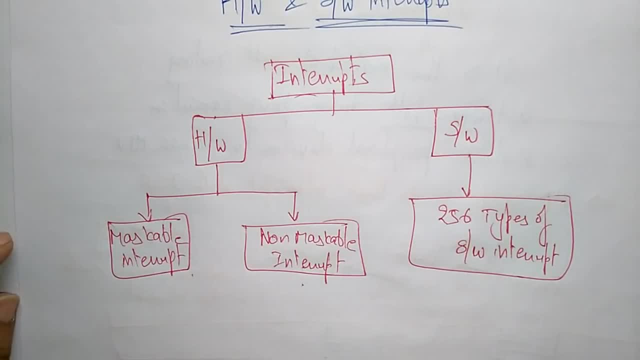 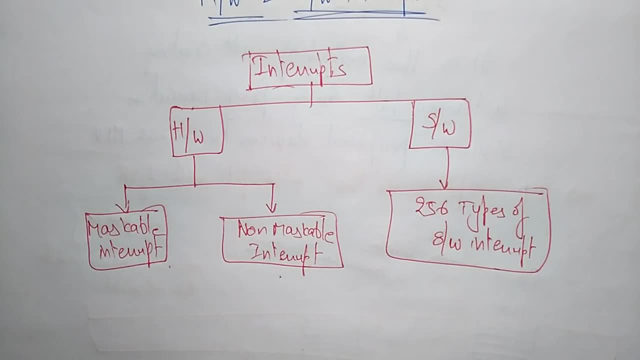 request and later it has to continue with the main program and there are the software interrupt. there are total 256 types of software interrupts. will be there for the non-maskable interrupts when the present. so actually this hardware interrupt caused by any peripheral devices. so whatever the peripheral devices that are connected to the processor, so this hardware interrupt caused by. 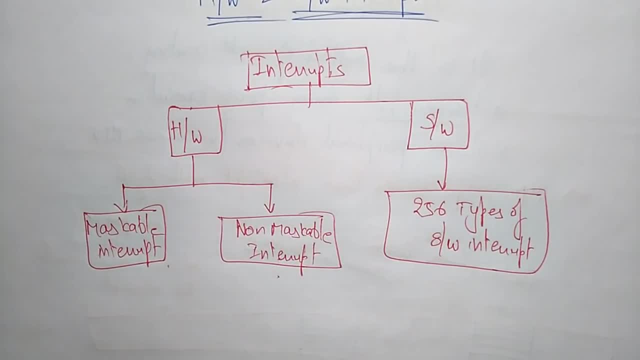 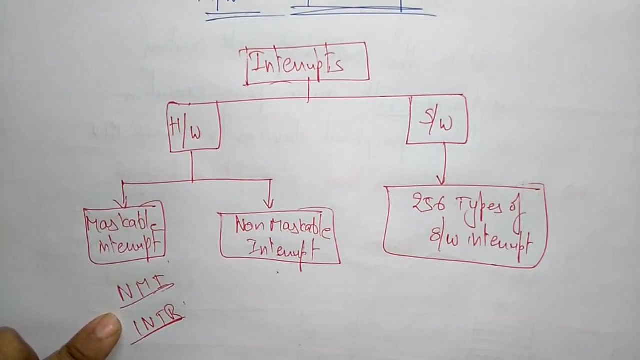 any peripheral devices by sending a signal through a specified pin to the microprocessor. so by using nmi, non-maskable interrupt or intr, by using these two pins. uh 8086 has two hardware interrupt pins, so these two are the hardware interrupt pins, that is, a non-maskable interrupt. 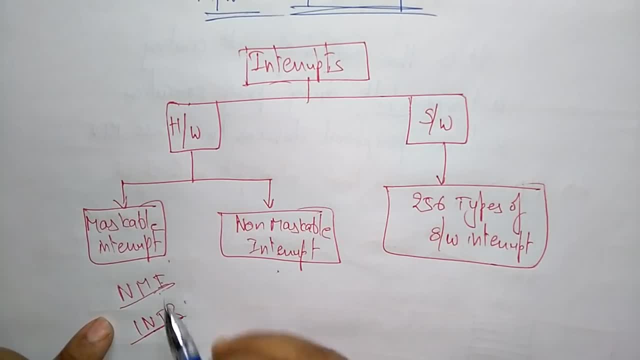 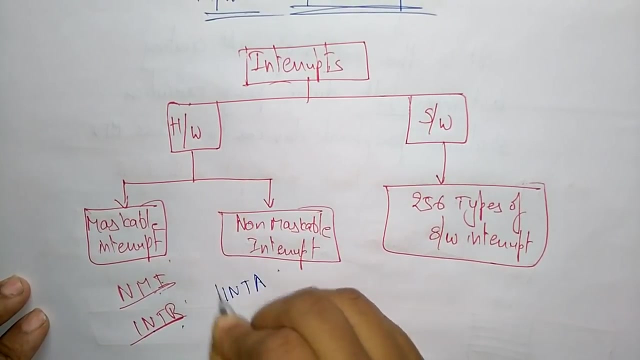 and intr. so whenever this non-maskable interrupt and intr uh is a maskable interrupt, having sorry non-maskable interrupt and intr is having a lowest priority. so one more interrupt pin associated with this, that is inta, so which is interrupt acknowledgement. so these are different three. 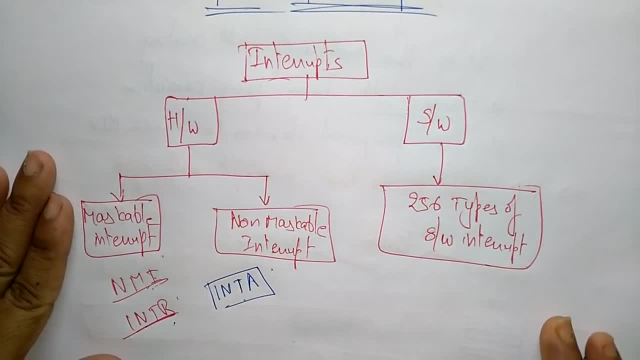 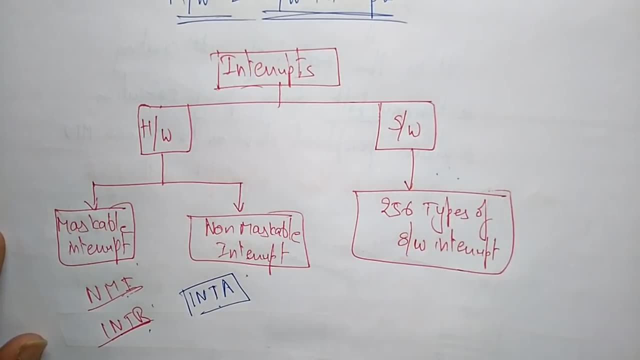 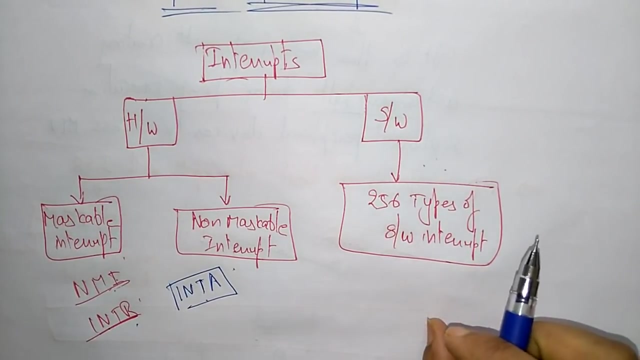 hardware pins that are present interrupt pins that are present in the 8086 microprocessor. now coming to the software interrupts, some instructions are inserted at the desired position. so whatever you are writing the program, so in the program some instructions are inserted at the desired position into the program to create an interrupt. so these: 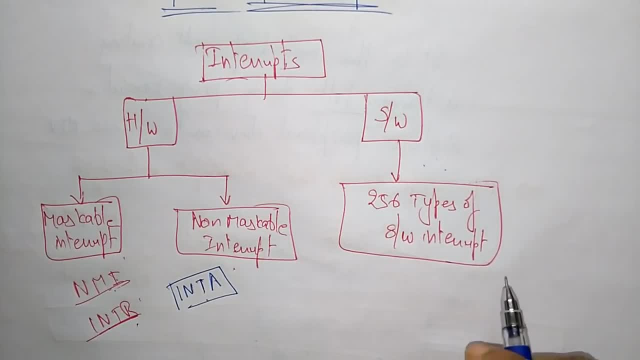 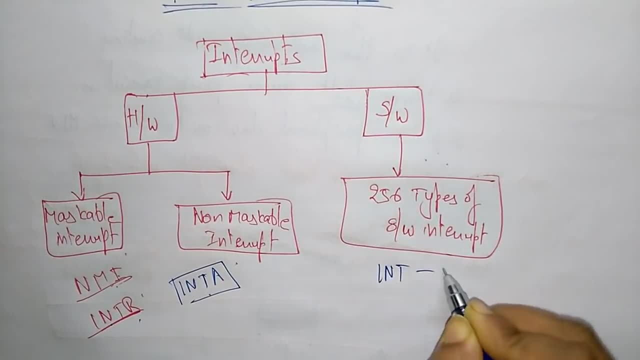 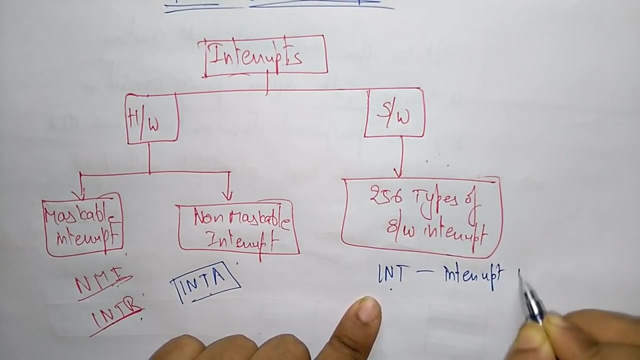 interrupt instructions can be used to test the working of various interrupt handlers. so those or int int is nothing but so. this is an instruction that is written in the program. int int indicates the instruction with the type number. you have to just mention the type number by interrupting the.